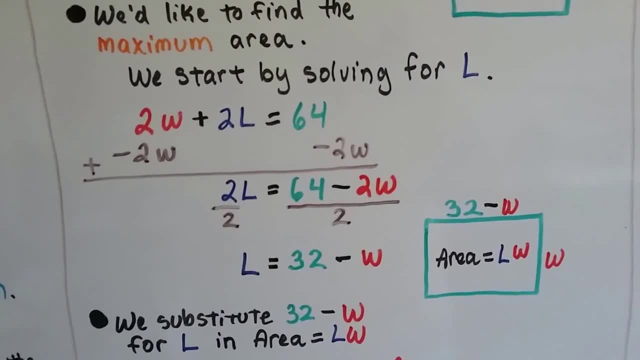 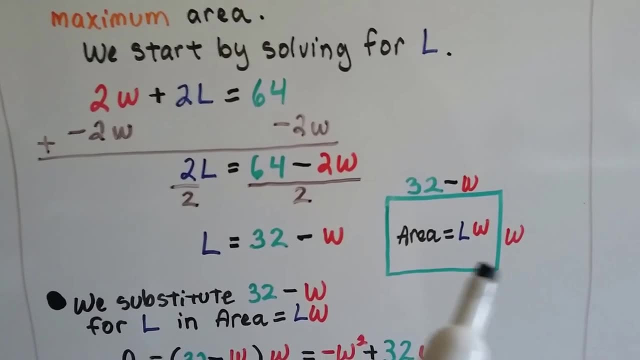 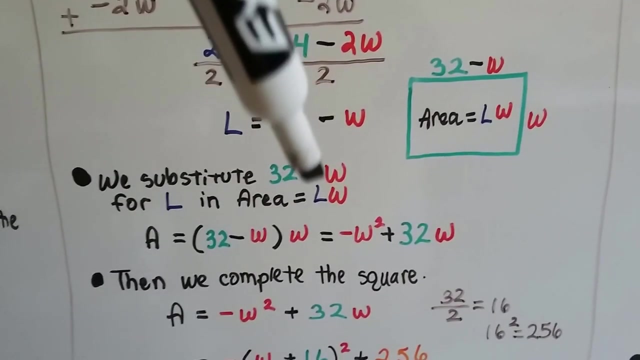 L equals 32 minus W. So now we can use 32 minus W for our L value. So we have 32 minus W times W is going to give us the area. So we substitute the 32 minus W into this formula- length times width and we get: the area is equal to 32 minus W times W. 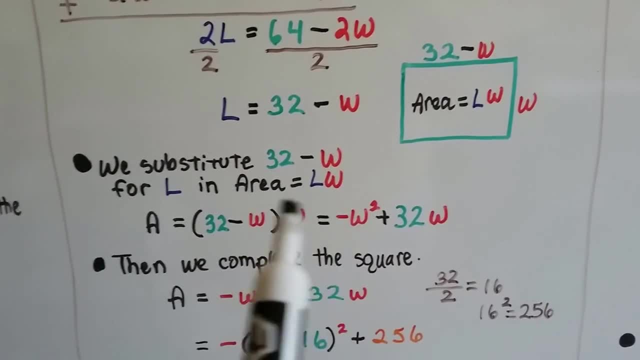 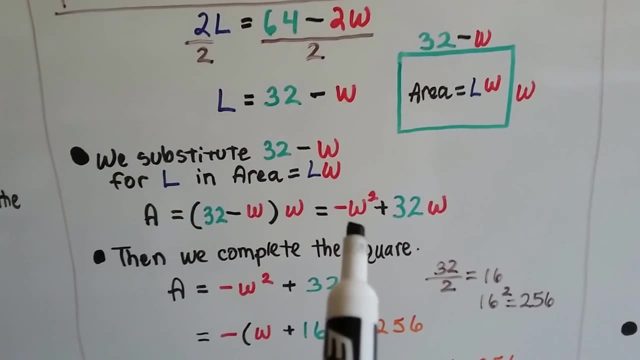 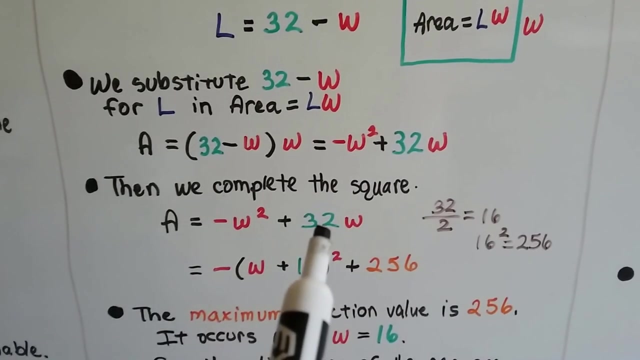 We can distribute this W, can't we? We're going to get a negative W squared with these two, and then we're going to get a 32W by distributing it over there. So now we have negative W squared plus 32W. All we have to do now is complete the square. We divide this value right here. 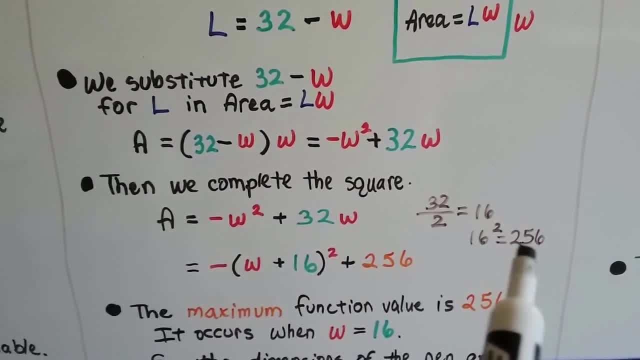 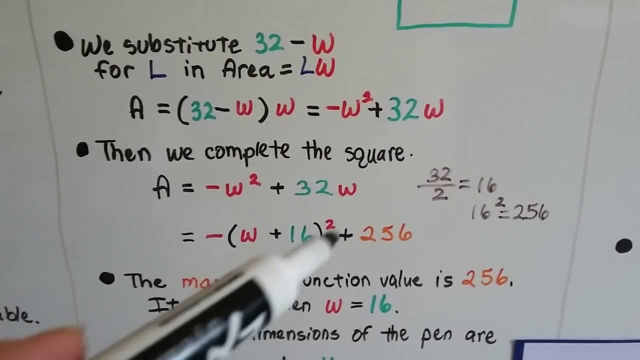 in half, We get a 16, and then we square it and we get 256.. So now we have a negative square of W plus 16 plus 32W. We return squared inultans 16 plus 32W plus 16.. So there's a two plus two叫256由256. 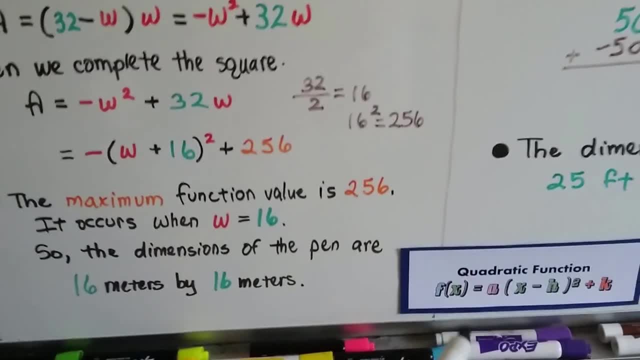 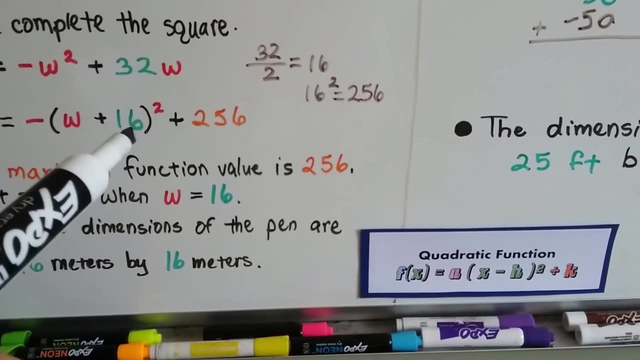 in that quadratic form. See, There's a two plus two叫256減256.. And there's a two plus two叫256減256. here's our A value, Right here it's an invisible one. Here's our X, here's our H, squared and 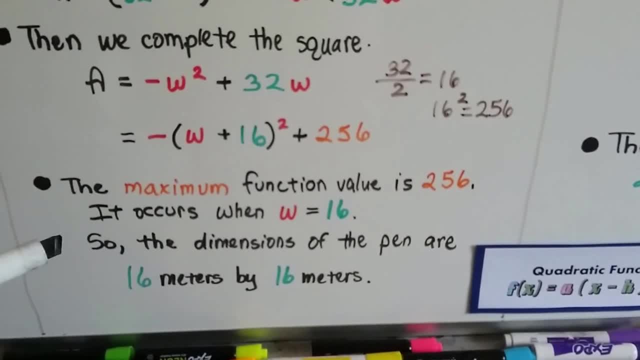 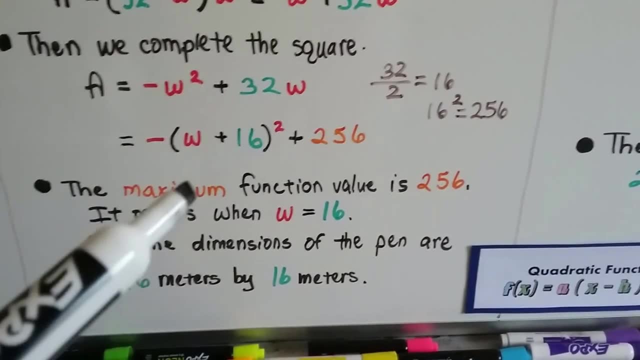 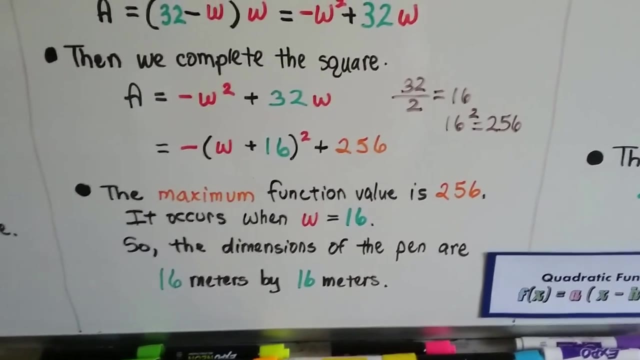 here's our K value: 256.. So the maximum function value is 256, this K value right here. And it occurs when W equals 16 and the dimensions of the pen are 16.. 16 meters by 16 meters. I know it said rectangle, but a square is basically a rectangle, It's got. 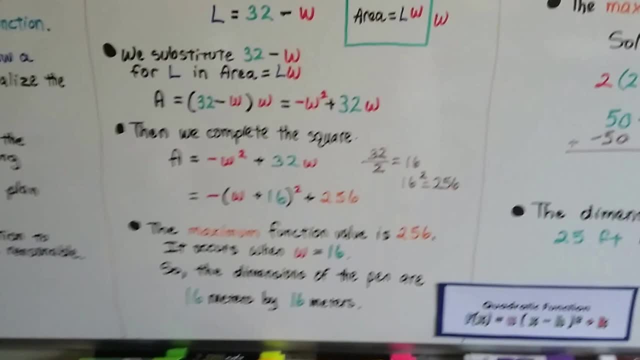 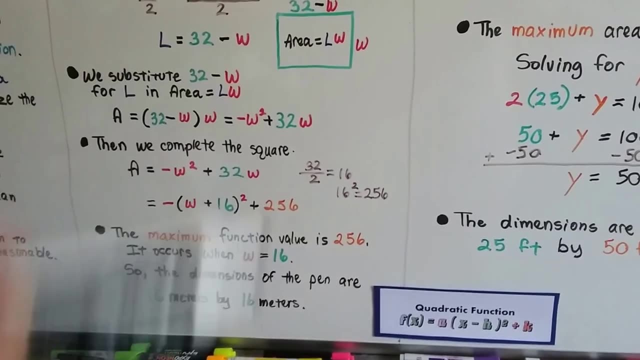 four sides, right, So be careful if that happens to you. okay, Don't think that it has to have one value larger than the other. 16 meters by 16 meters would still be a good answer for that. all right, Makes sense. Let's try another one. We've got another fencing problem. We've got 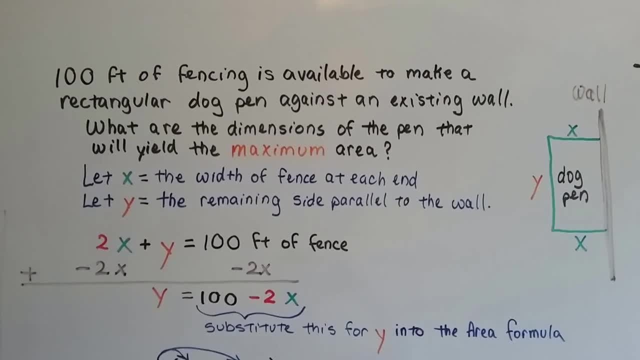 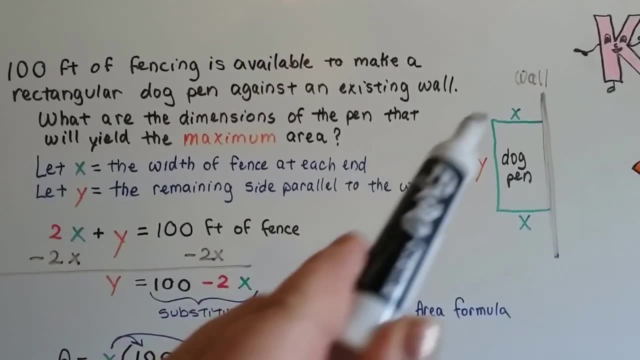 100 feet of fencing is available to make a rectangular dog pen against an existing wall. So here we have this existing wall of a building. We've got 100 feet of fence. so all we need is three sides, don't we? Because that wall is going to make the other side. So what are the dimensions? 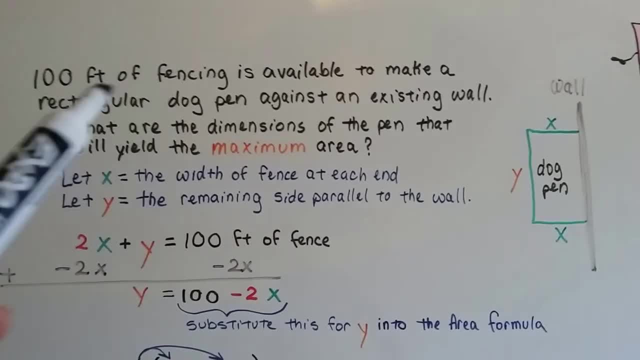 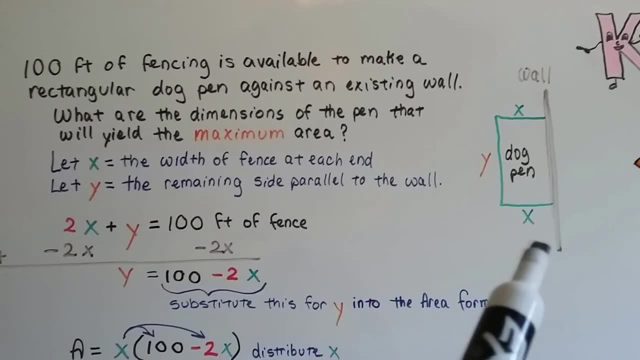 of the pen that will yield the maximum area. What's the largest dog pen that we can make with that 100 feet of fencing? So we're going to let the x equal the width of the fence at the ends and the y is going to be the remaining side, parallel to the wall. So now we have two x's. 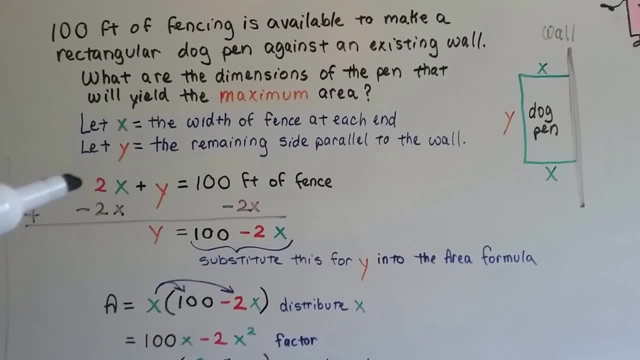 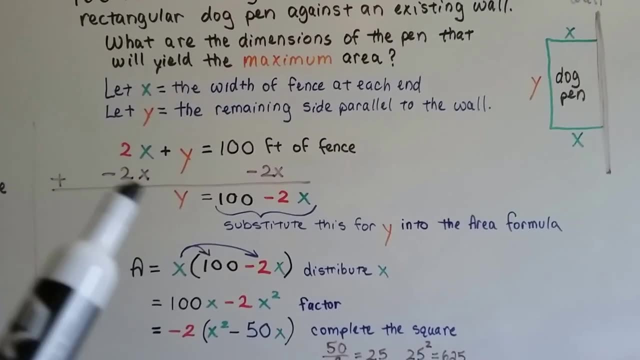 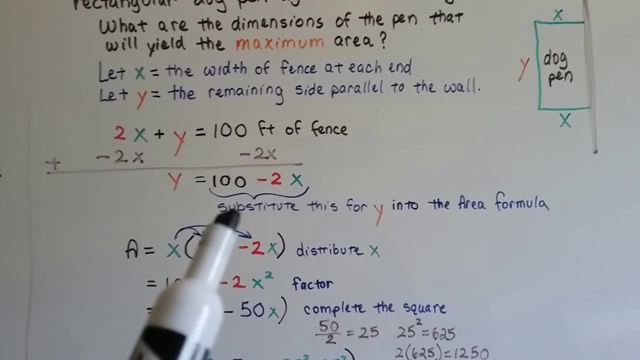 plus a y, don't we? Two x plus a y? y equals 100 feet of fence. We can add a negative 2x to each side of the equation so we can isolate y and we get y equals 100 minus 2x. Now we could substitute this for y into the area formula 100. 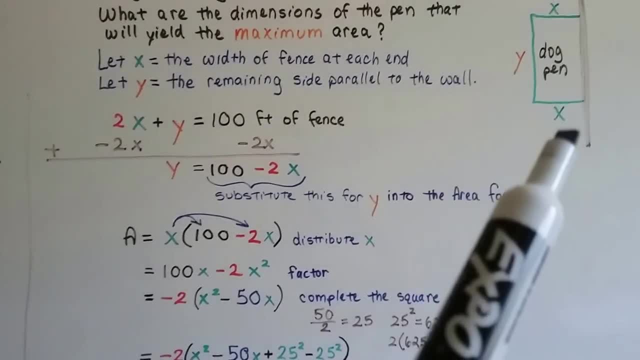 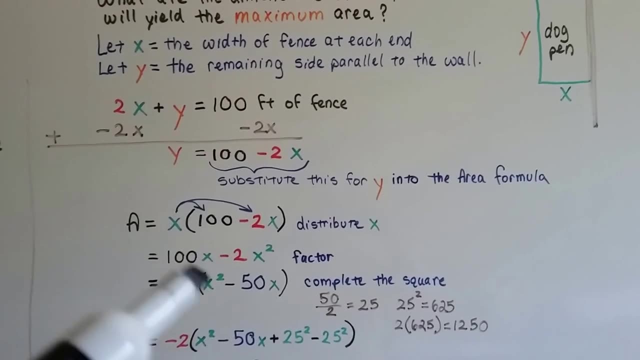 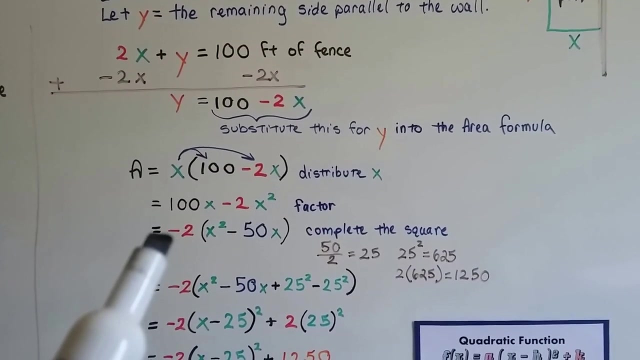 minus 2x. So instead of x minus y we've got x minus 100 minus 2x. We can distribute this x and we get 100x minus 2x squared. We can factor this: We get a negative 2 times x squared minus 50x. 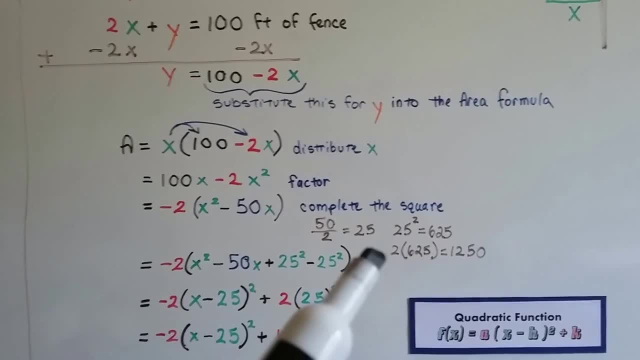 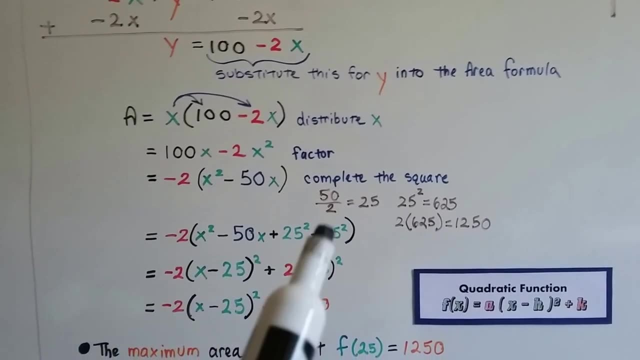 We can complete the square. We divide this 50 in half and get a 25, and then we square it 25 times 25 is 625 and we can add it inside the parentheses like this, and then take it out. We can split this, can't we? 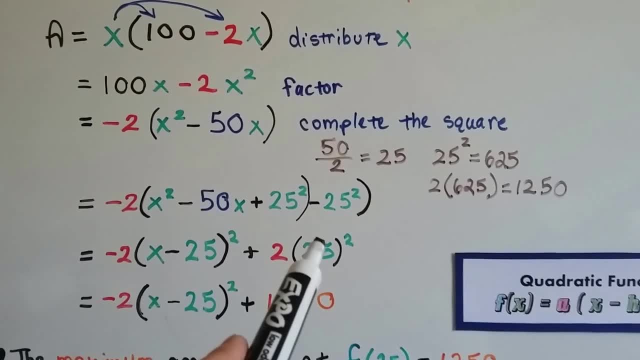 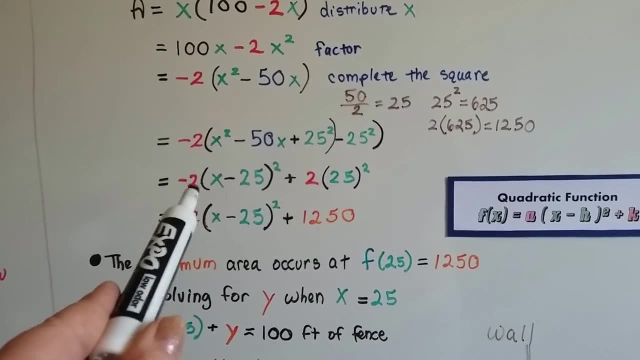 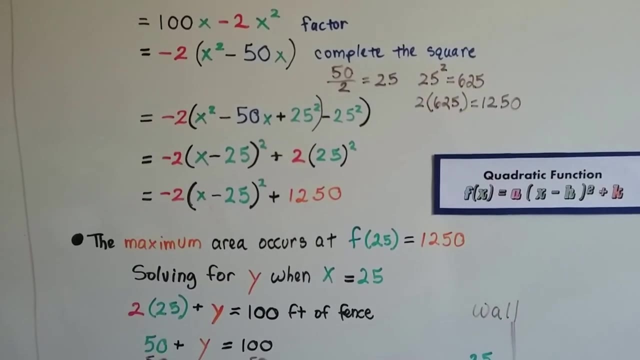 We can split. this can go like this, like we did in the last couple of videos, and we can add this: 25 squared, just like this, and now we have a negative 2 times the square of X minus 25 plus 2 times 25 squared. now, if you're really confused, you need to see the last. 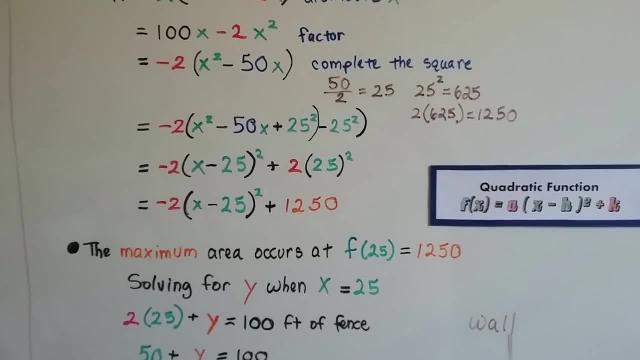 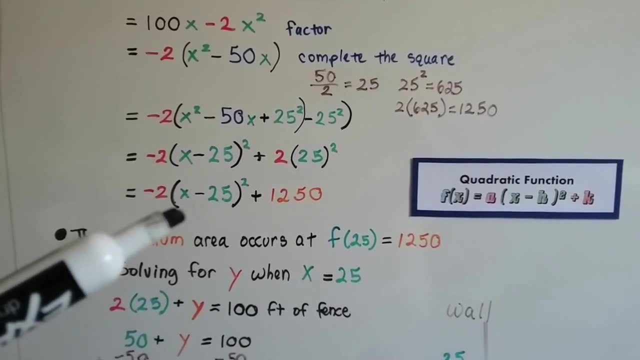 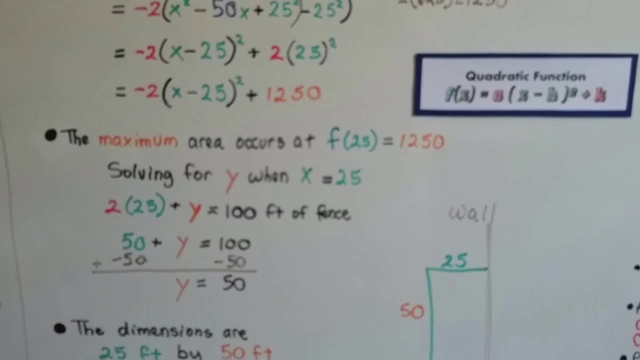 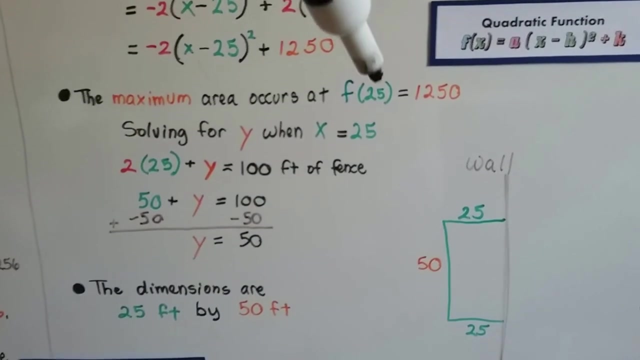 couple of videos, 9.5 a, B and 9.6 a. that'll really help you. we've got negative 2 times the square of X minus 25 plus 1250. that's our K value. the maximum area occurs at the function of 25 equals 1250. that's our X value. seeing: 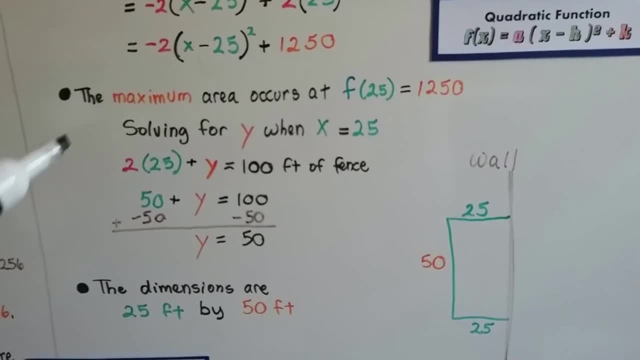 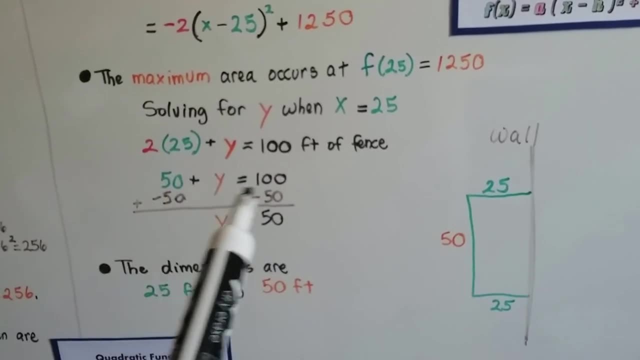 solving for Y. when X equals 25, we get 2 times 25 plus Y equals that hundred feet of fence. that means 50 plus Y. we can add a negative 50 to each of those and that's our K value. so that's our K value, so that's our. 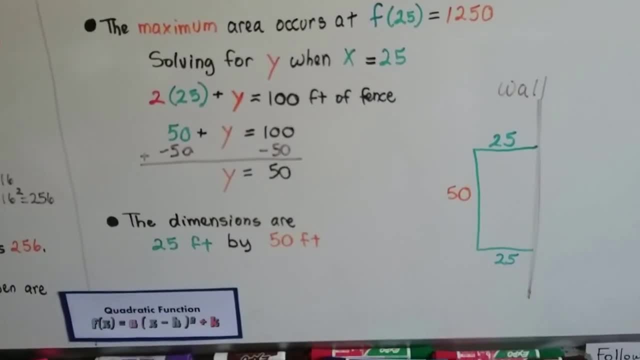 Y and Y is 50 minus 15 is our K value. so that's our K value, so that's our Y. and we add to our Y and we get 24.5.. We add from each side to isolate Y, we get Y is 50. so 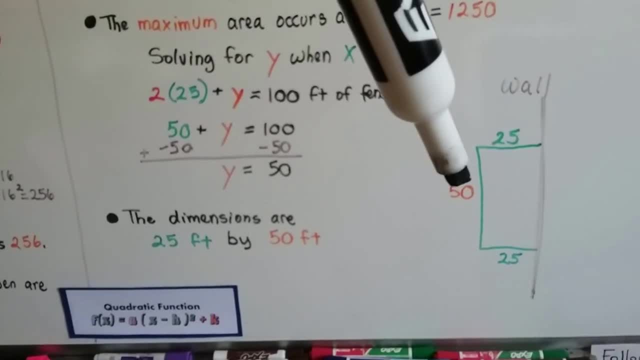 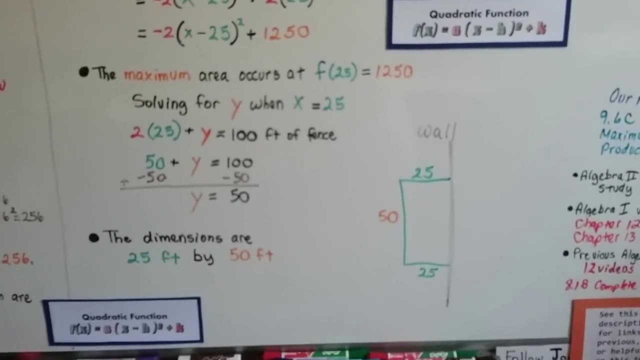 we know the dimensions of the fencing will be 25 feet by 50 feet. See how I did that. So, like I said, if you're really confused you have to go back and watch the last couple of videos, and there's going to be links in this description. so